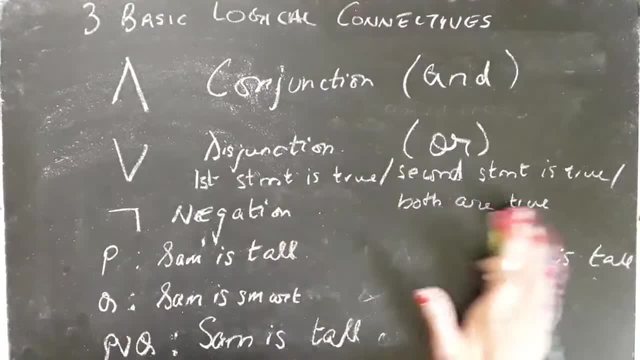 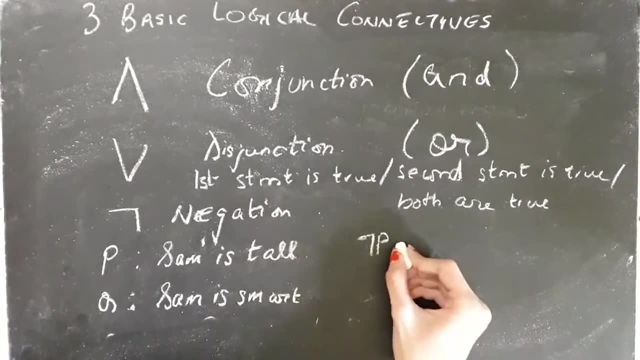 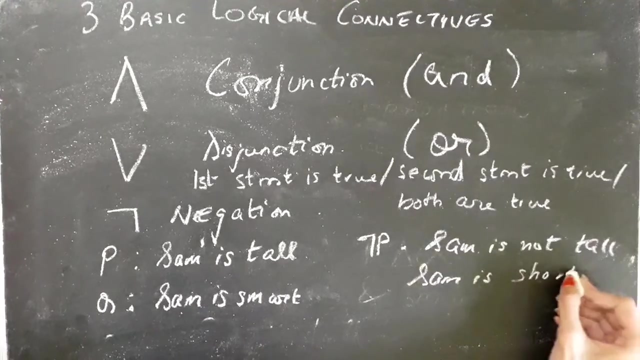 For example, in our example, what is the negation of the statement? P Denoted as negative of P? It is: Sam is not tall, or in other words, Sam is short. Okay, We can also have the negation of the previous statement that we had. that is negation of. 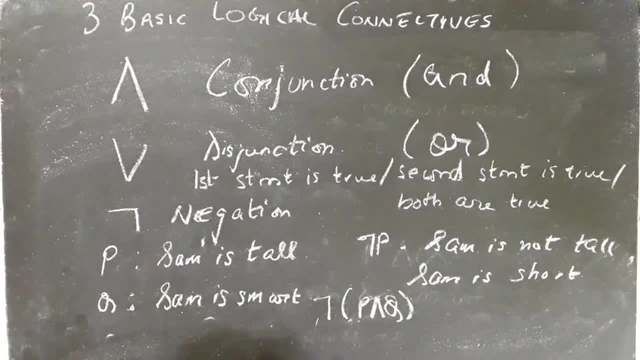 P and Q. What is the negation of P and Q? Sam is neither tall nor smart, So this way we have learnt the three basic logical correctness. Okay, Thank you, Bye, Thanks. Those are our common connectives in 빠이�BI. 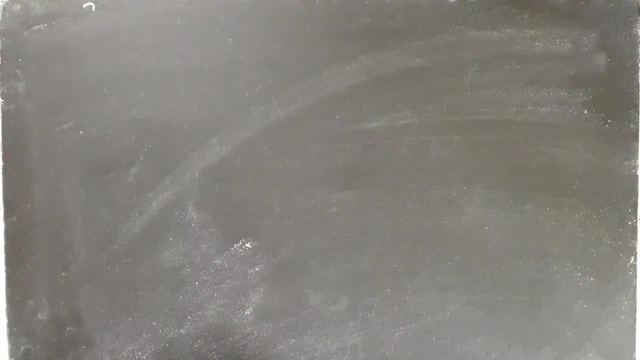 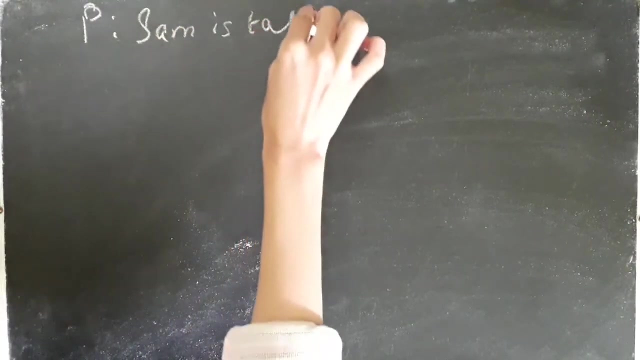 Now we move on to truth tables. What we need to understand is that every propositional sentence has either a truth value or a false value. For example, let us again consider: Sam is tall. If it so happens that Sam is indeed tall than the truth value of the statement is true. 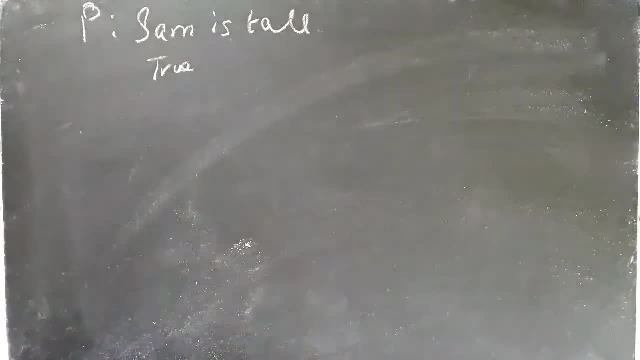 and if he is short than the truth value of this statement is false. There cannot be any difference. So that means the Durable stands for logруз지 and 중정 İ Qnasta 이 충분히 이� sevent sy inconven 62 cândİr facts. 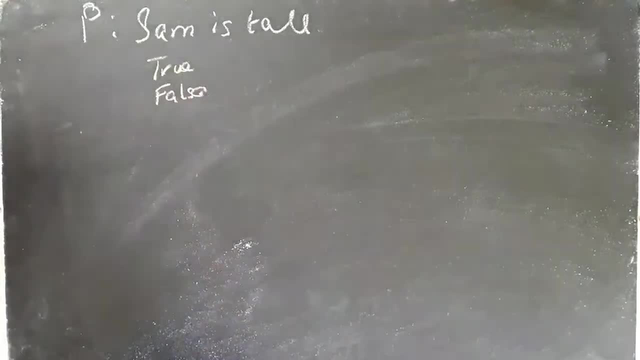 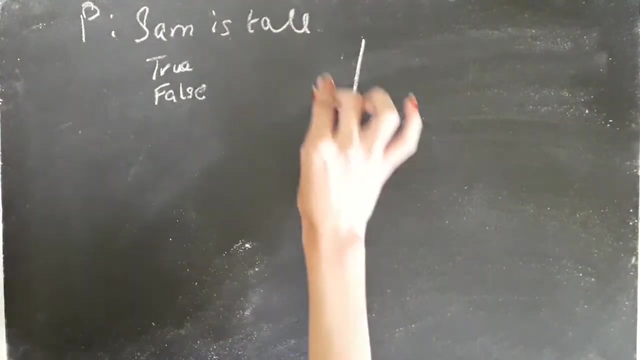 Though it may be that sometimes it may take our fault that the expression some other verb. Similarly, every propositional statement has a truth value which can be either true or false. With the help of these truth values, we can make the truth tables In truth tables. the basic truth table is that we write the propositional statement. 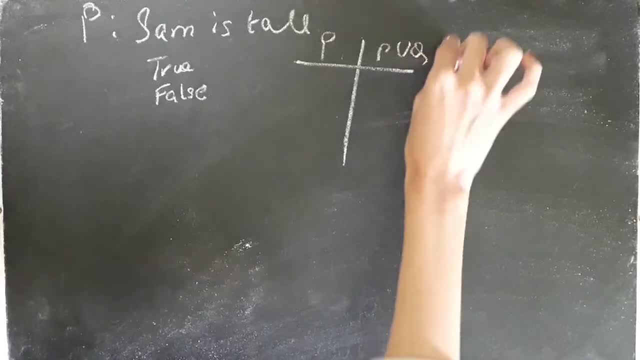 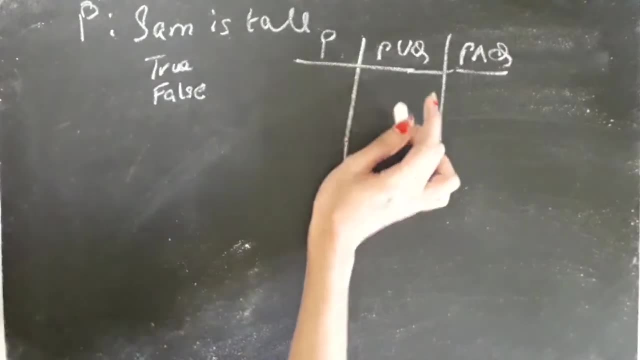 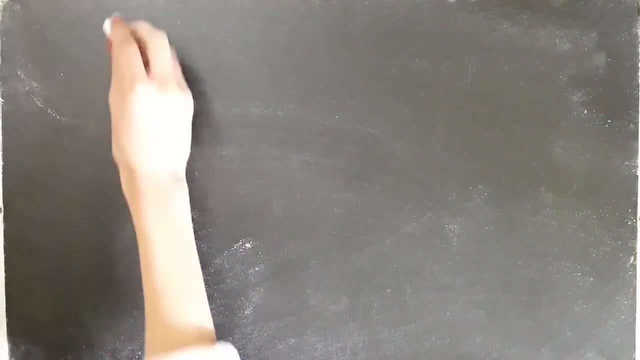 here say P, P or Q, P and Q, whatever we are asked to find, and we assign truth values to it. that is true, false, false, true. whatever be the truth value that we are given. Let us consider an example. 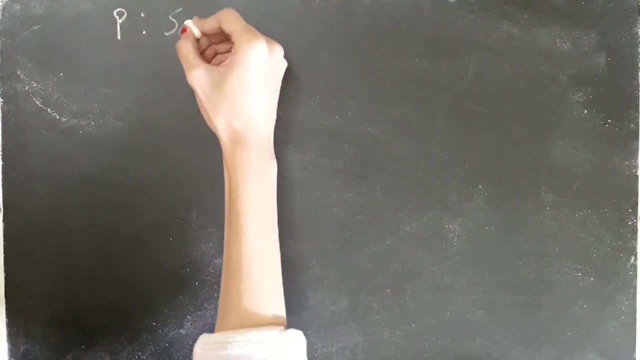 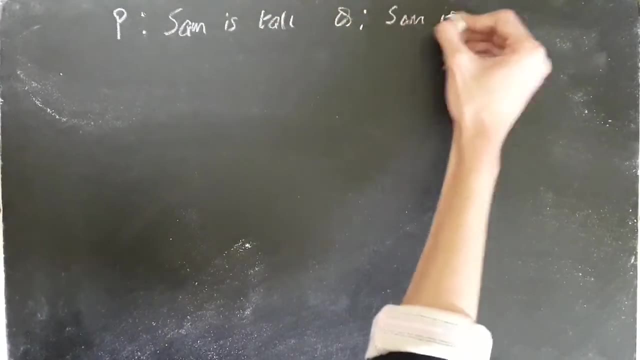 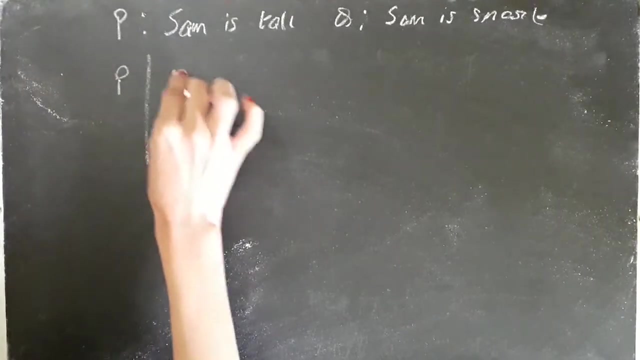 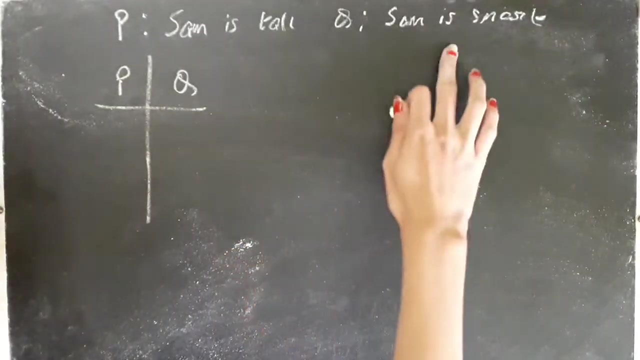 Let's again consider these two statements: Sam is tall and Sam is smart. What will be the truth value of these two statements together, not singly? If we are considering them as two single statements, then the truth value is true, false and true, false for both. 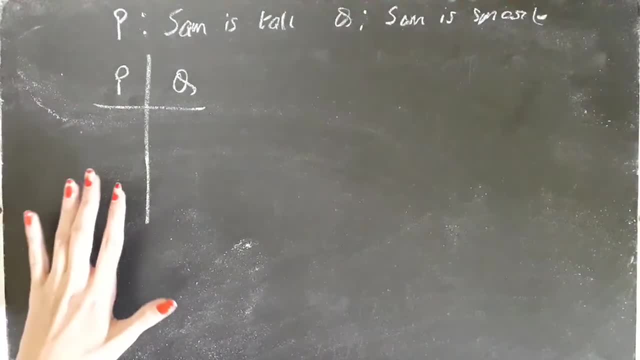 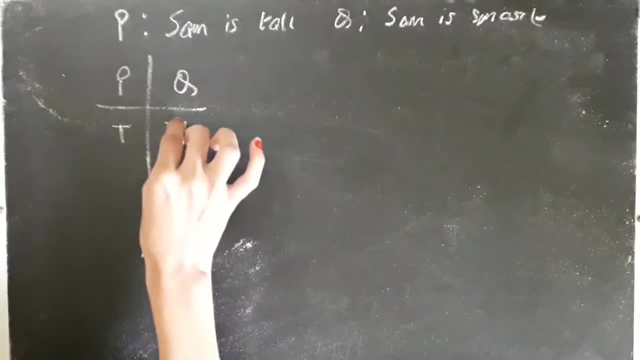 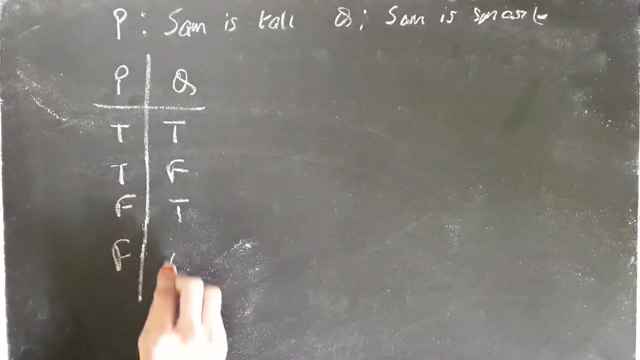 these statements separately, But if we are considering them together, then what are the possible truth values that we can assign them? It is both of them can be true together. one can be true, the other false, which can happen in two ways, or both are false together. that is, Sam is tall and smart. 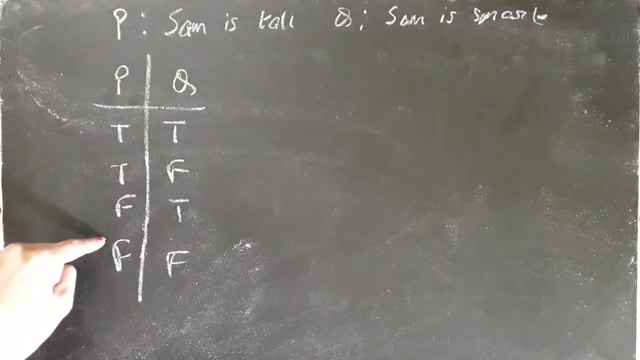 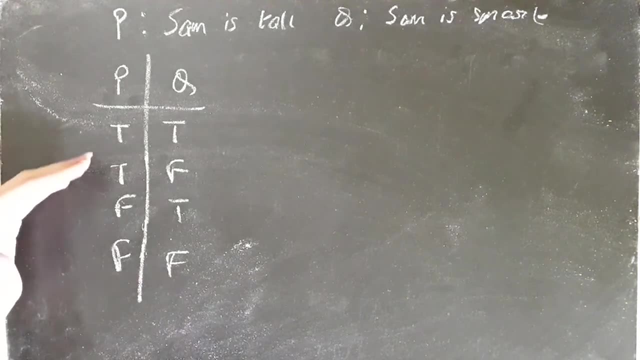 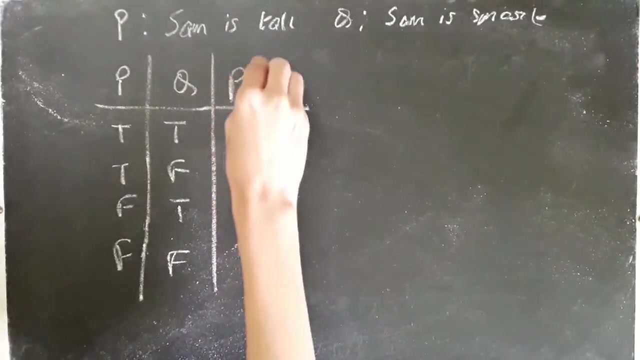 Sam is tall, but he is not smart. Sam is not tall but he is smart. Sam is neither tall nor smart. So these are the truth values that these two statements can be assigned together. Now suppose we have to find the truth value of the statement P and Q. 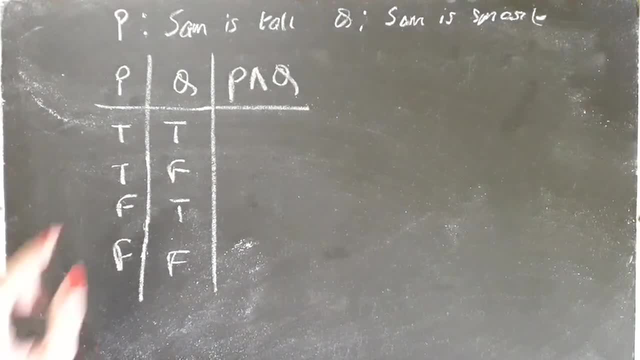 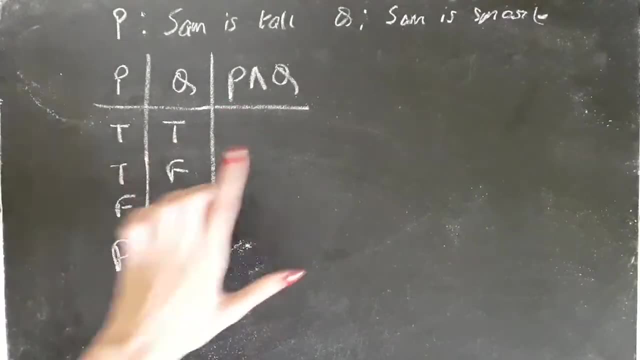 For P and Q to be true, it is necessary that both these statements are true together. Here we see that P is true and so is Q. Thus, P and Q are also true In this case. P is true and so is Q. 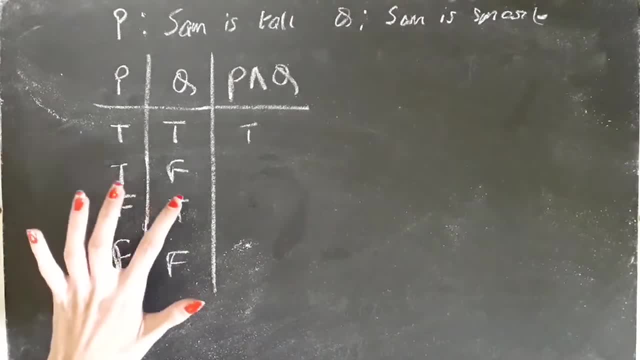 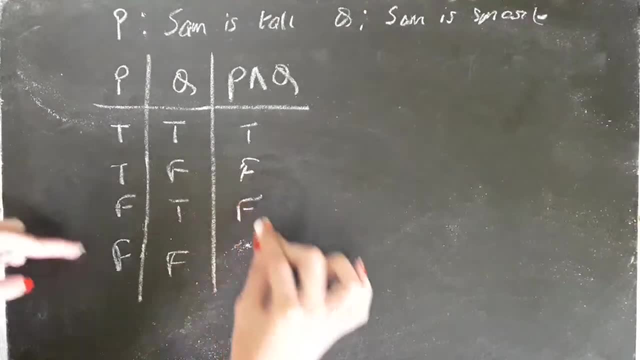 In this case, P and Q are also true. In this case, P is true, but Q is false. Thus our statement P and Q becomes false in this case. Similarly, it is false here, and obviously it is false here as well, because none of the 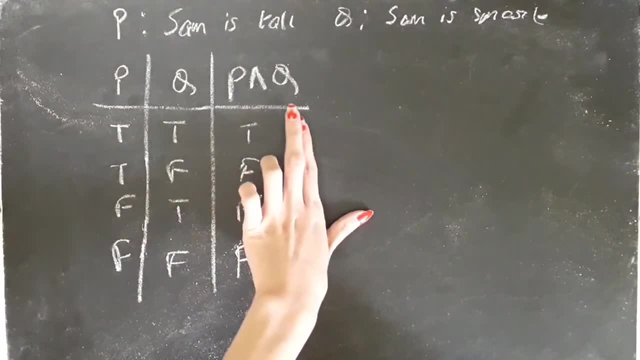 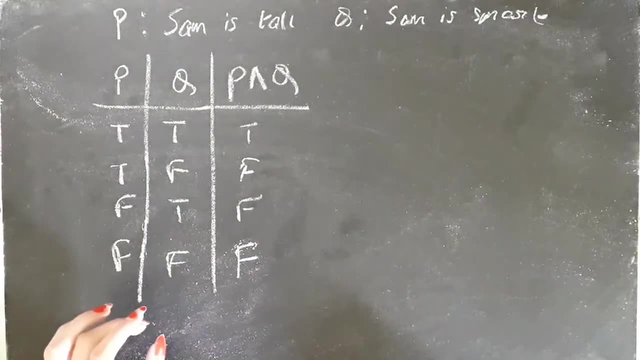 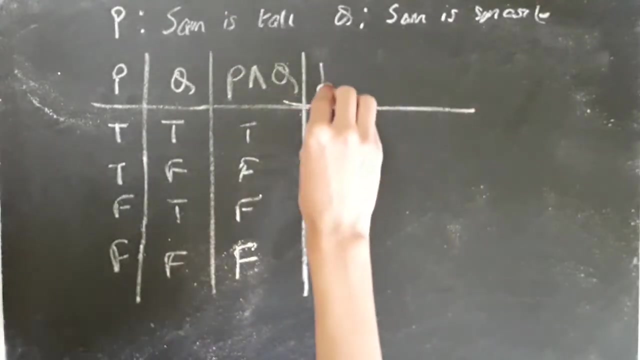 statements are true. Thus we see that for the conjunctive logical connective to be true, it is necessary that both the statements that make up the conjunctive statement should be true. Otherwise, in all other cases it is false. Now, if we are to consider, 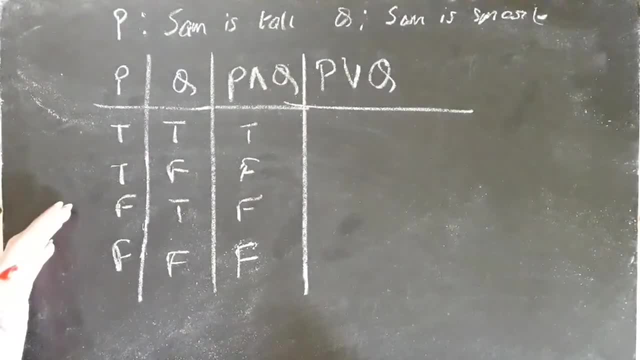 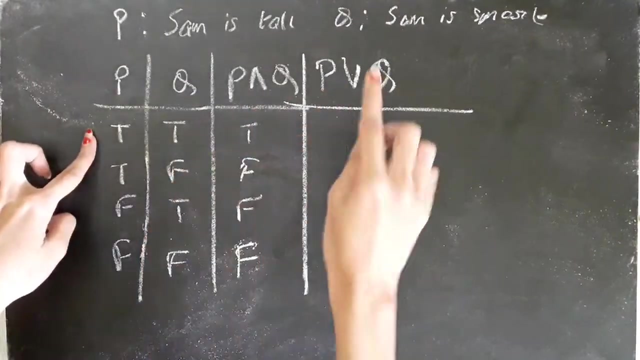 Consider the truth value of P or Q. Remember that we had learnt that for P or Q to be true, what is necessary is that either one of the statements should be true or both of them should be true together. So in the first case, both of them are true together. hence P or Q is true. 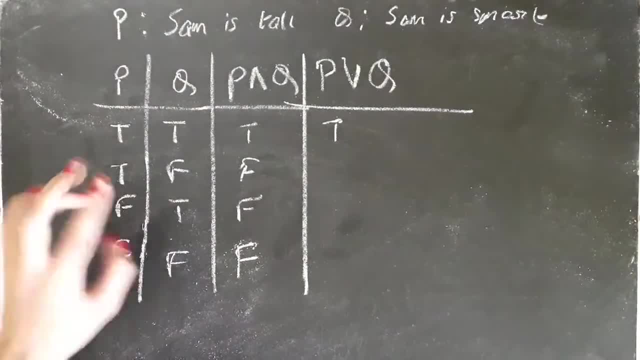 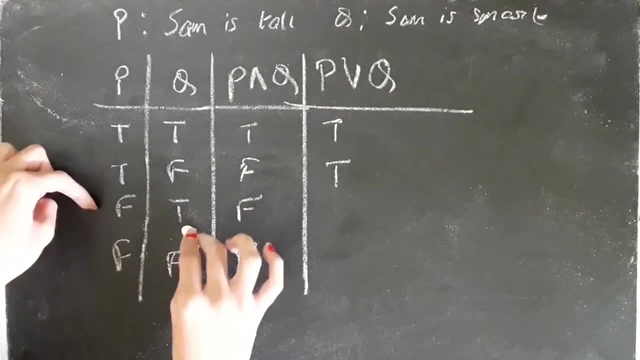 Here P is true, but Q is false. However, only one statement's truth value should be true is necessary. So again this is true. Similarly, here Q is true. so this is true as well, but here both of them are false. So P or Q cannot be true. 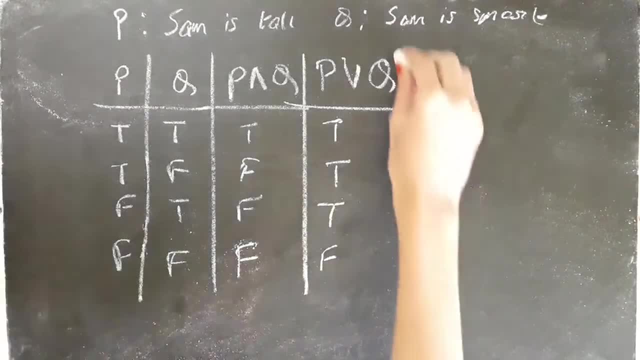 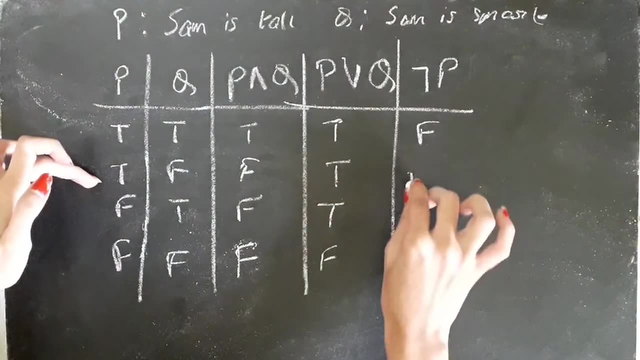 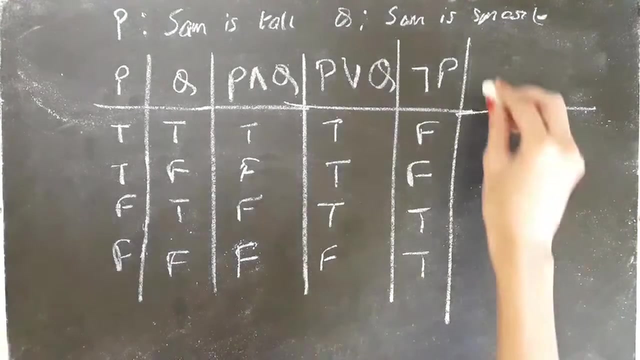 So it is false. Now what is the negation of P? Just reverse the truth values and we get negation of P as F, F, T, T. Now suppose we have to find the truth value of the statement, not P or Q. 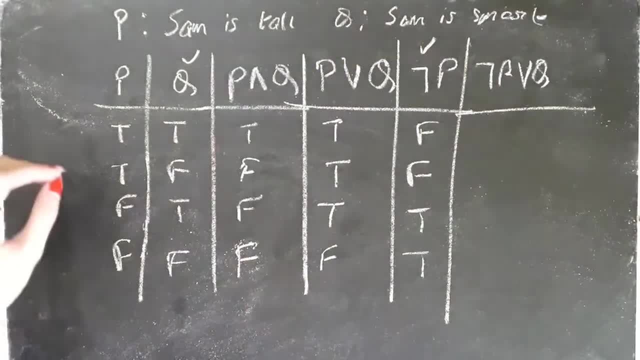 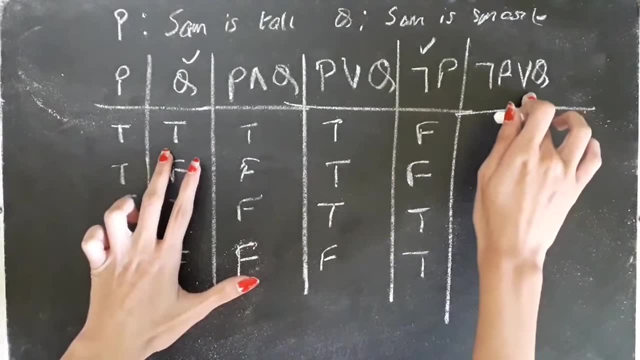 That is, we need to consider these values as well as these values. So we see T and F. So the disjunctive logical connectives condition is satisfied because one of them is true. So not P or Q is true in the first case. 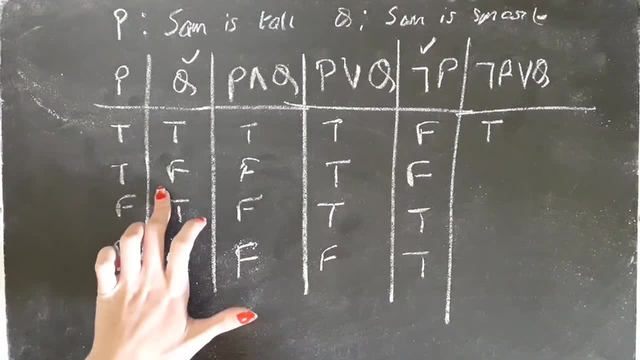 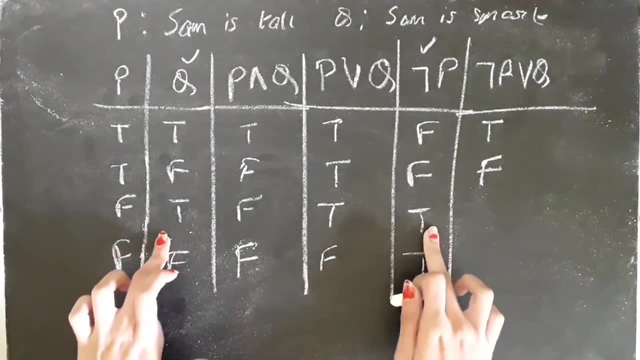 In the second case, both of them are false. So obviously the condition is not satisfied. and it is false again Here. both of them are true together. So not P or Q is also true. And in the fourth case this is false. but this is true. 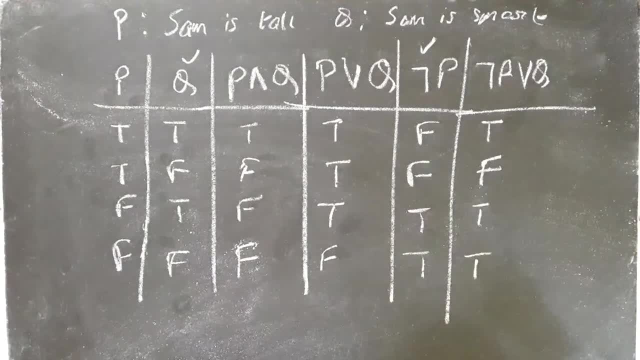 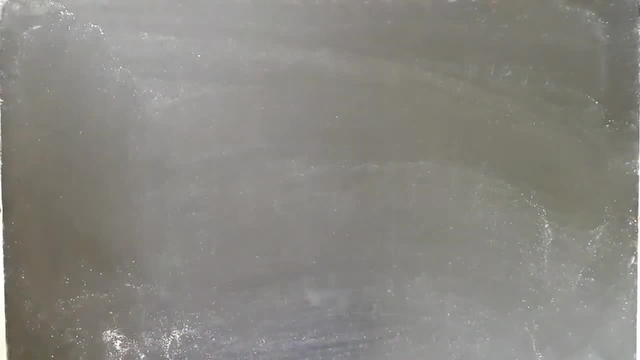 So again, this is satisfied and we get a true value here. So this is how we make truth tables. We can have truth tables for a variety of logical connectives, And now we move on to tautologies and contradictions. What is a tautology? 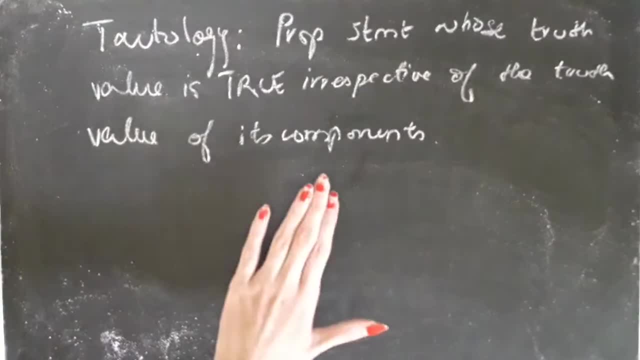 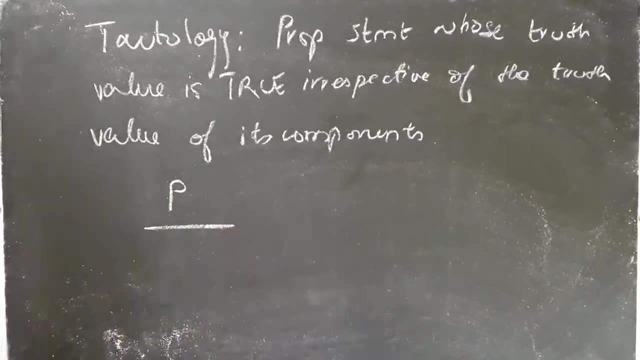 A tautology is a propositional statement whose truth is true. The truth value is true irrespective of the truth value of its components. For example, let us consider a statement P. The two truth values of P are either true or false. Now let us consider negation of P. What is negation of P? 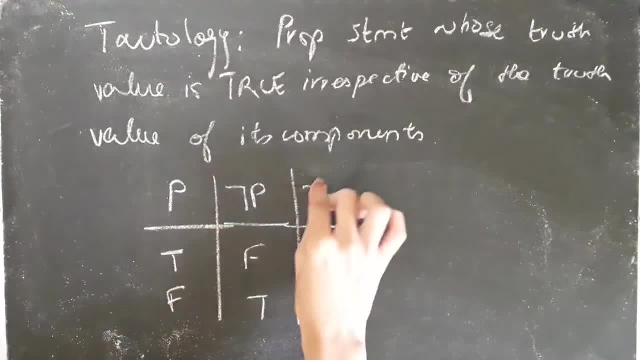 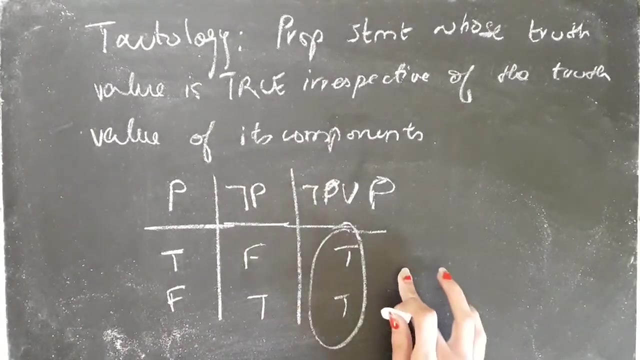 It is false and true. Now, if we are to find not P or P, what is the truth value of this statement? It is true, true. So we say that this statement- not P or P- is a tautology, because its truth value is always. 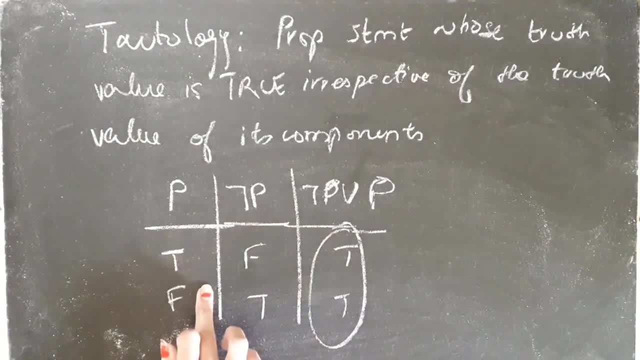 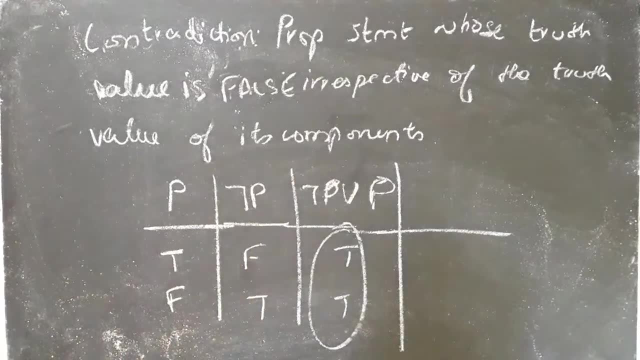 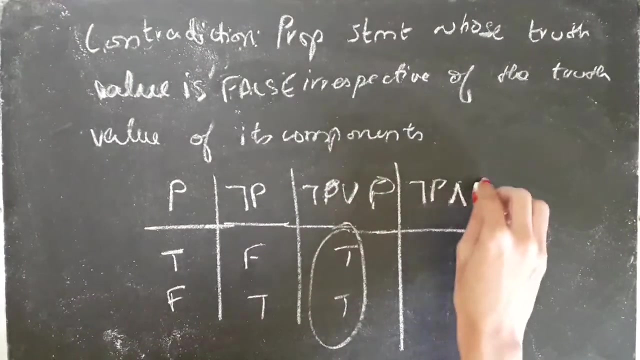 true, irrespective of the truth value of its components. You see that. So here we have a tautology That means the truth value of a contradiction is always false, no matter what be the truth value of its components, For example, negation of P and P. What is the truth value of this? 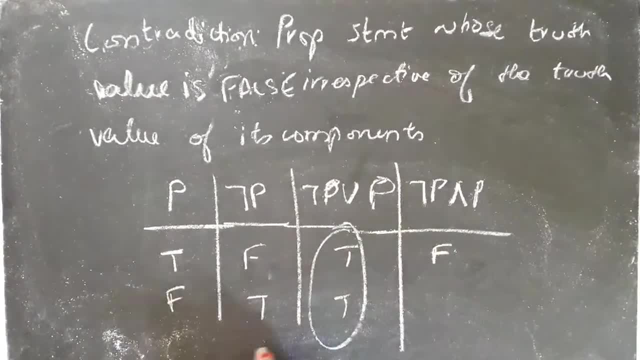 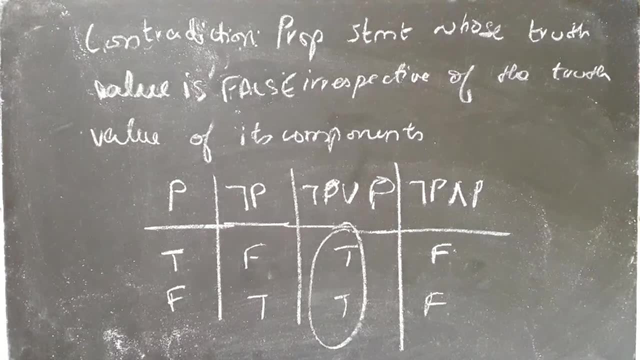 For the first one it is false. For the second one it is true. And for the second one also it is false. Hence its truth value is always false, no matter what be the truth value of its components. Thus we see that it is a contradiction. 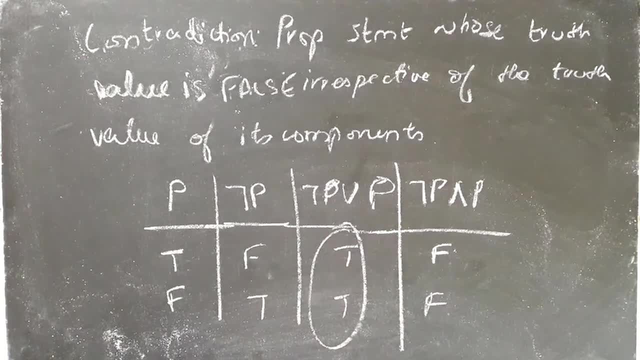 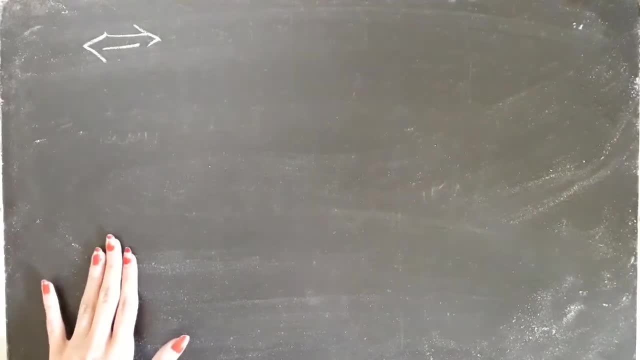 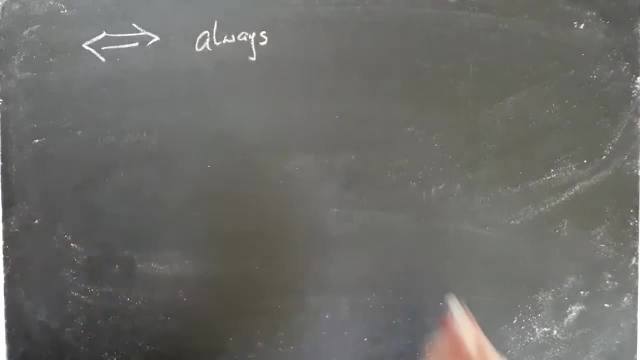 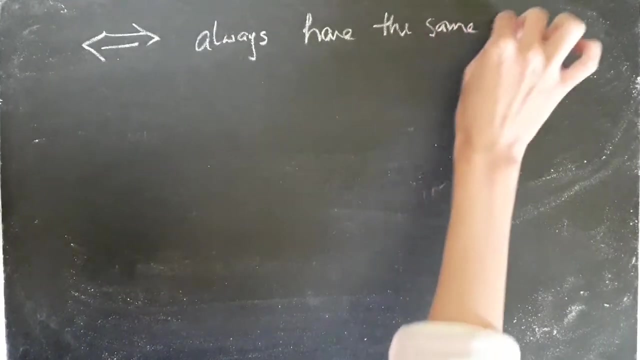 So these are contradictions and tautologies. Two statements are said to be logically equivalent if they always have the same truth value, irrespective of the truth value of their components. So what is the basic rule of identifying a logical equivalent? Logical equivalents always have the same truth value. 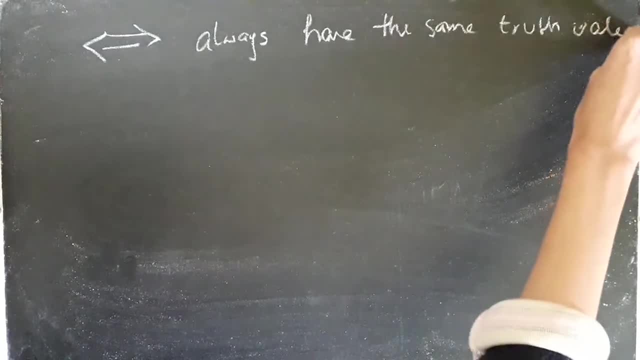 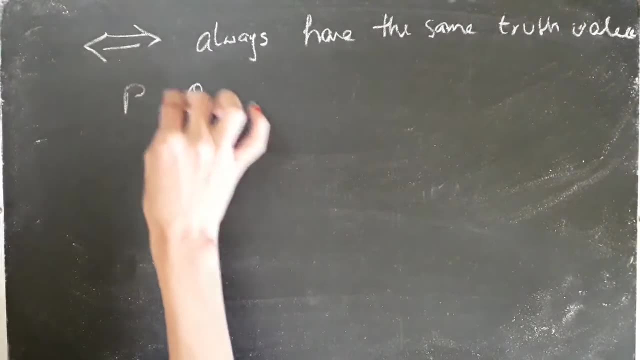 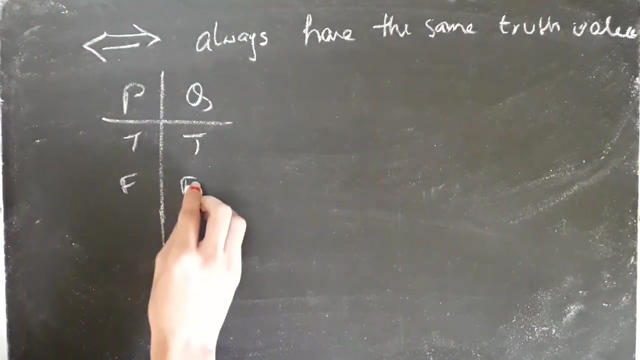 Now this truth value can be true or false. Let us consider an example. Let's consider PQ. Now, PQ can be true together, false together, Tf Ft. What is PQ? PQ can be true together, false together, Tf Ft. 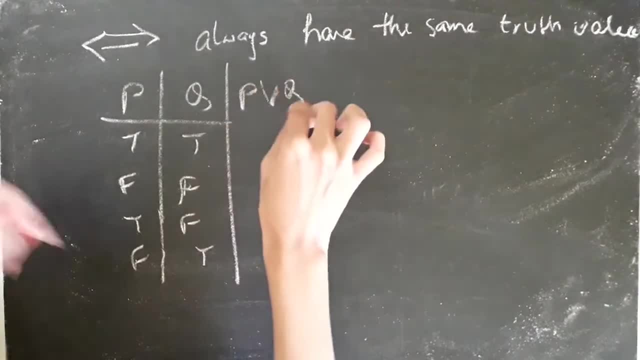 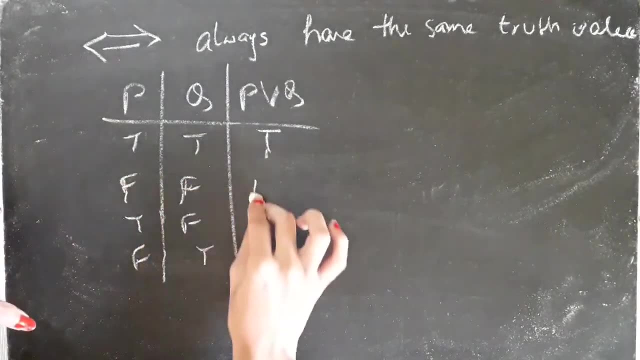 What is PQ? PQ can be true together, false together, Tf, Ft. What is PQ? PQ is P or Q? What is true together? So true, False together. So this will also be false. One of them is true. 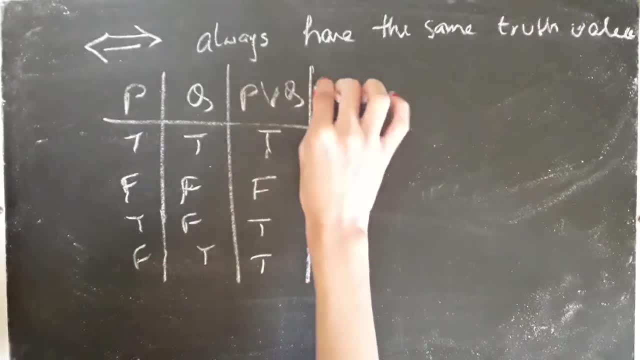 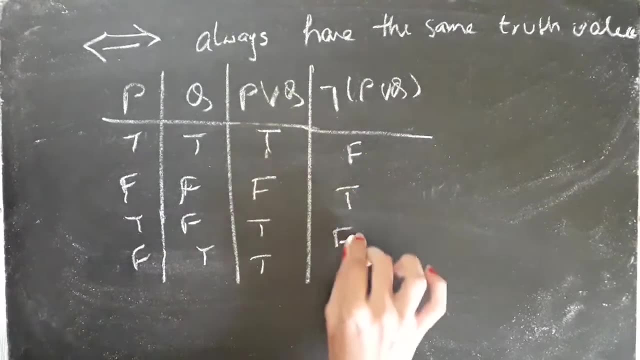 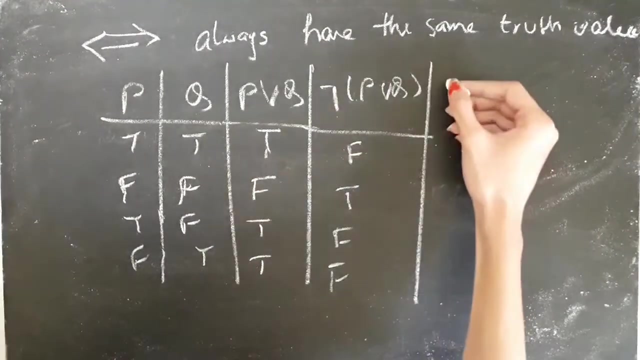 So it is true. Now, what is negation of P or Q? It is FT, F, F, Just reversing the truth values. Now, if we are to say truth here, Now what is true? It is true. if we have to find the negation of p, what is the negation of p? 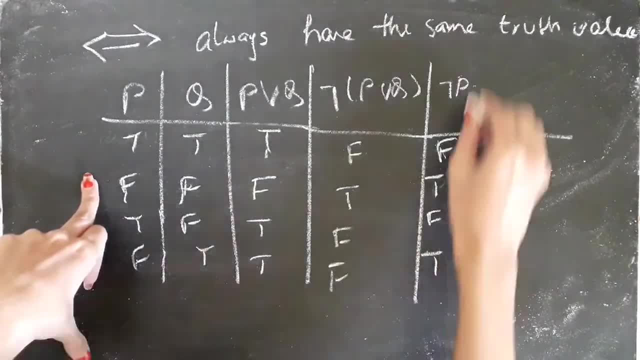 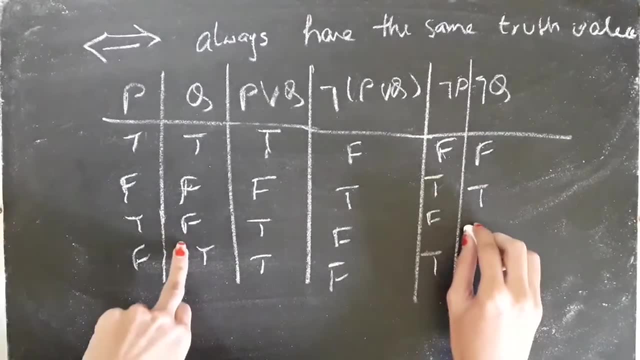 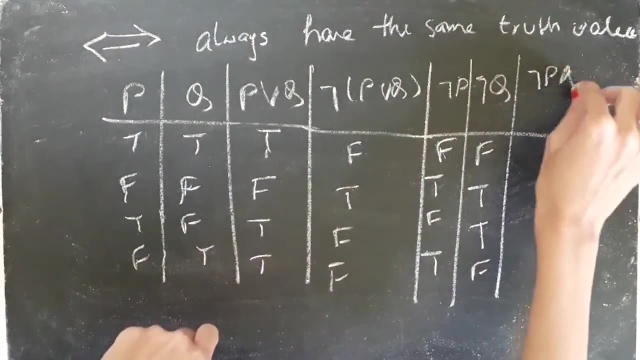 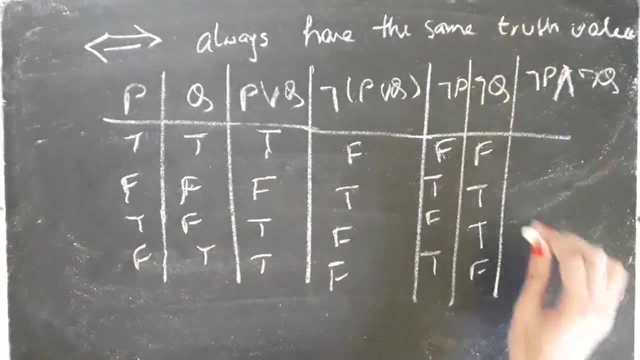 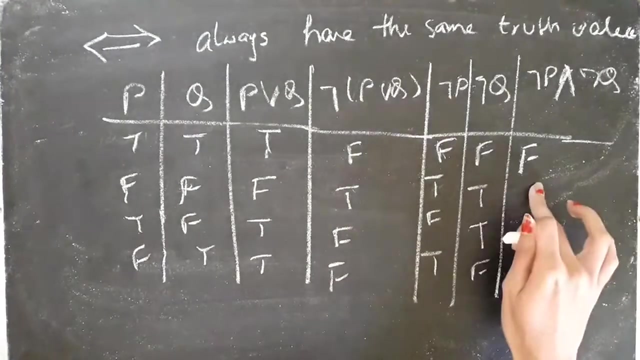 f, t, f, t. and negation of q is f, t, t and f again. now, what is negation of p and negation of q? q? it is, you see, that there is a conjunctive sign here. so both of them are false together. so the conjunctive connective is not satisfied and it is false here. both of them are true together. 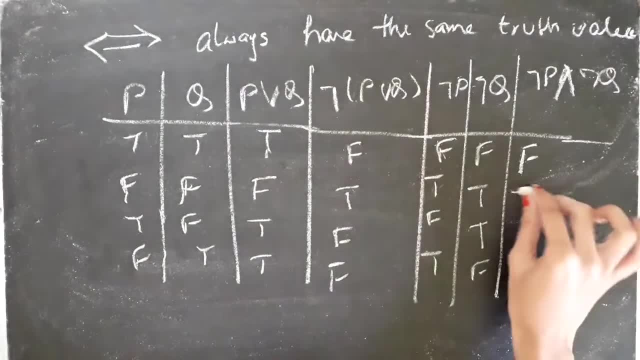 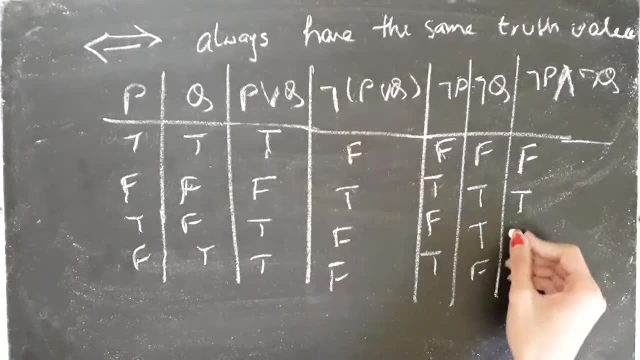 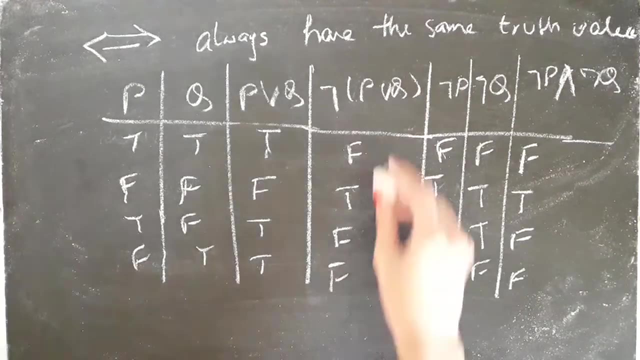 so obviously not p and not q are also is also true here. not p is false, but not q is true. thus they cannot be true together. so again it is false and similarly it's false in this case as well. now we see that the truth values of these two statements are same. whatever be the truth values,